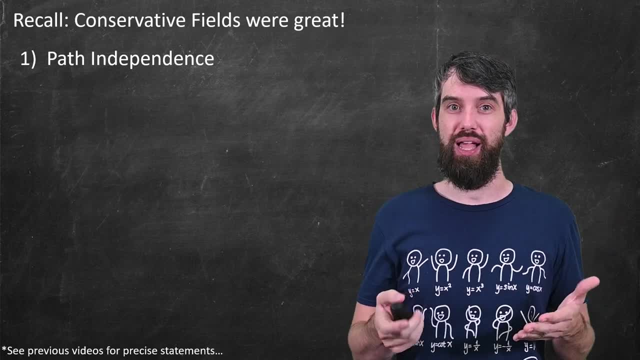 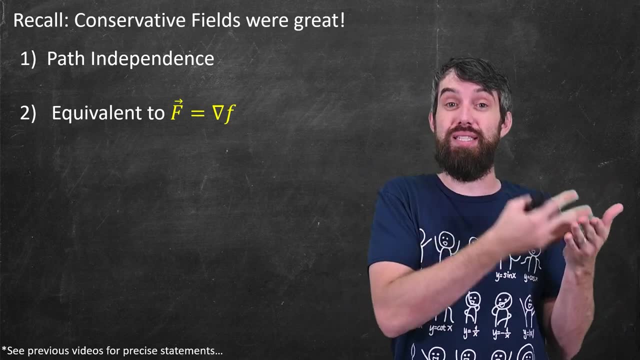 all that matters is the endpoints for a particular line, integral. Second of all, they were really nice because we saw that they were the equivalent to the field being able to be written as the gradient of some scalar potential function: little f. And then, thirdly, 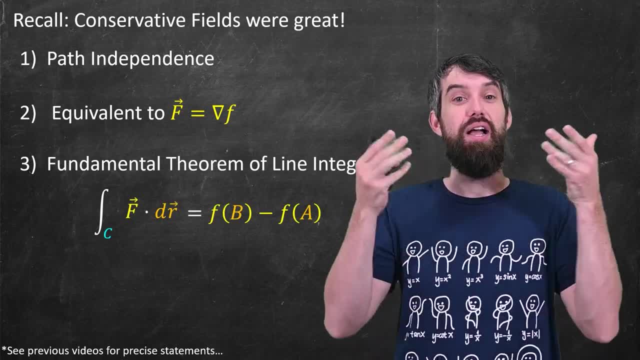 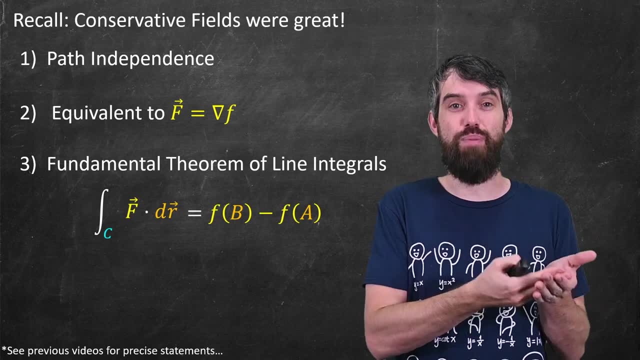 we saw that the fundamental theorem of line integrals applied to conservative fields and it said that the line integral of f dot dr was just written as the difference between the function at its endpoints f of b minus f of a. So for these reasons, conservative fields are: 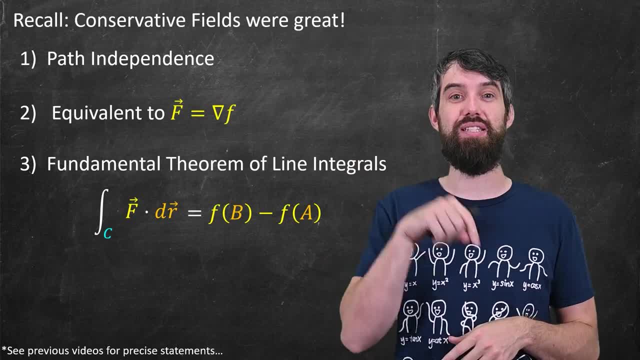 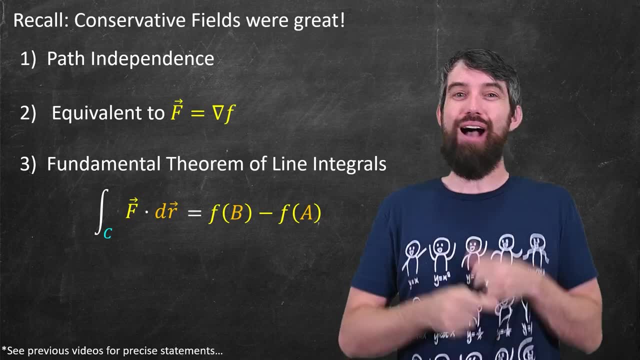 very nice And we've seen all of this in more detail previously on our vector calculus playlist. the link for that is down in the description. But I have some questions. First of all, how do we know if a field is conservative? I mean I can like it? 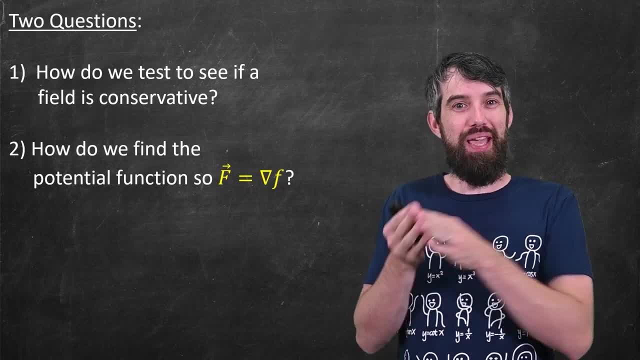 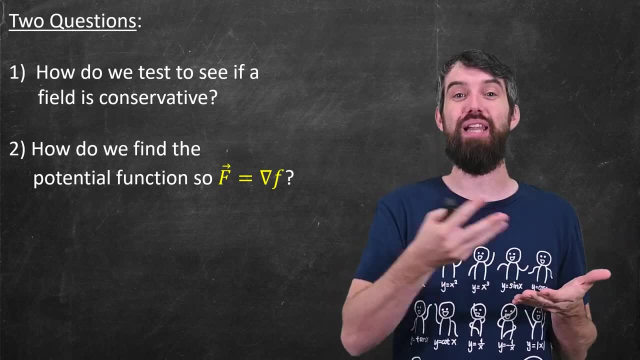 but how would I know? And in particular because the definition of a field being conservative is that it's independent of a path. I don't want to go and compute infinitely many different paths. That sounds like a lot of work. So I want to come up with a quick way to look at a field and to know. 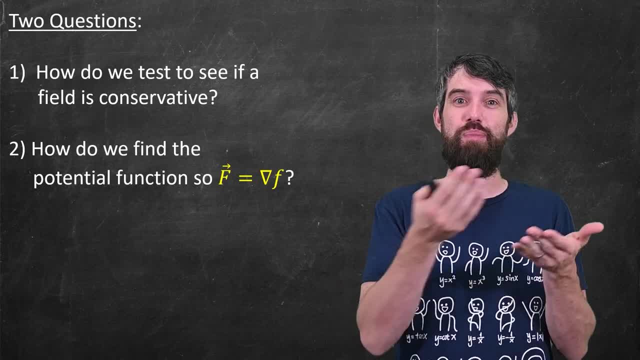 whether or not it is conservative. And then, second of all, because being conservative implied that you could write it as the gradient of a potential function. well, what's that function? How do I find it? And then, thirdly, because being conservative implies that you could write it as the gradient of a potential function. 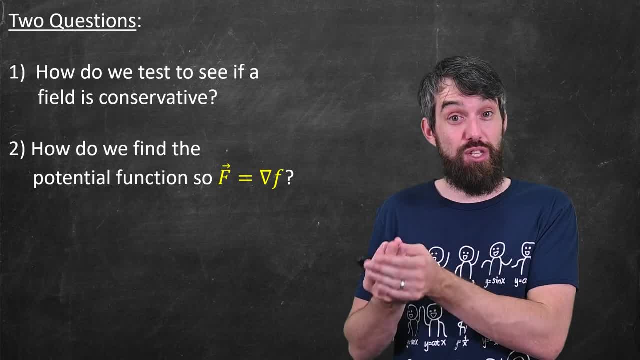 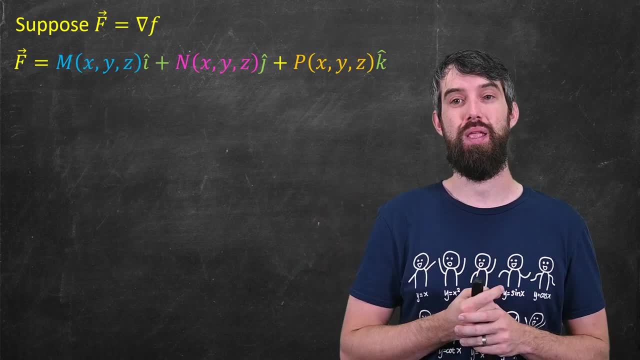 how do I find that little f? So I have two different questions. I'm going to take up the first of these questions in this video and the second in the following video. Suppose that I've got my f and it's written as the gradient of a potential function. Well, I'm actually going to give some name to the. 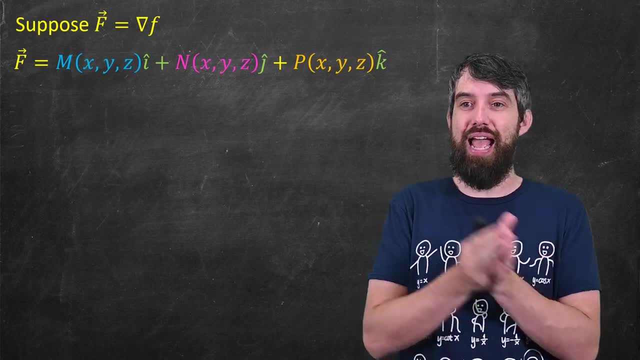 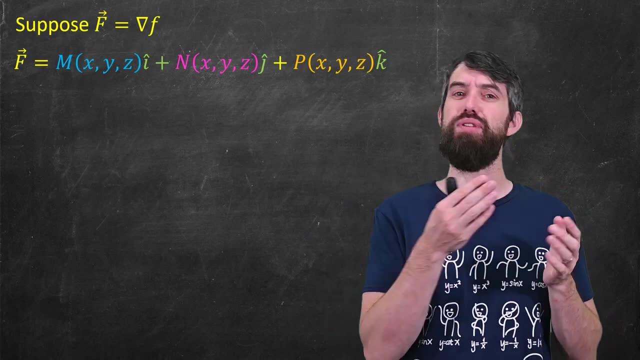 components. I'm going to say in three dimensions that my field f can be written as an m in the i hat, an n in the j hat and a p in the k hat. I'll try to be consistent with using m, n and p in. 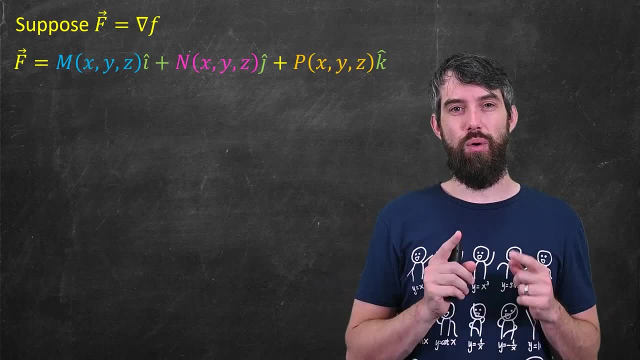 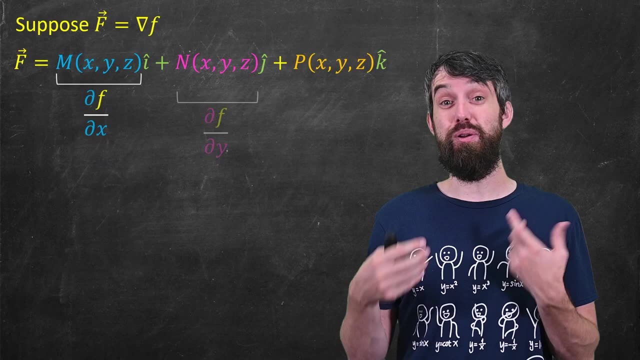 this way every single time when I've got a three-dimensional field. Now, because of the assumption that this can be written as the gradient of a scalar potential function, this means that each of these components can be written in terms of little f, So the m is just the partial of f, with. 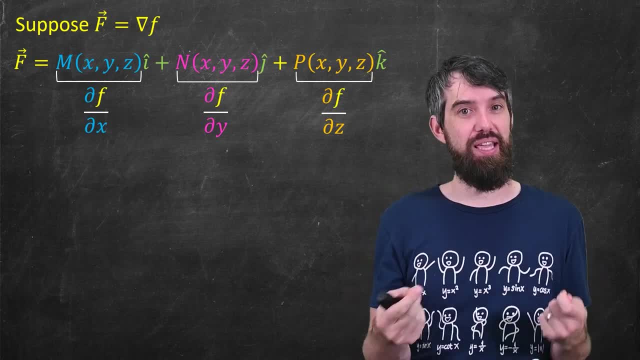 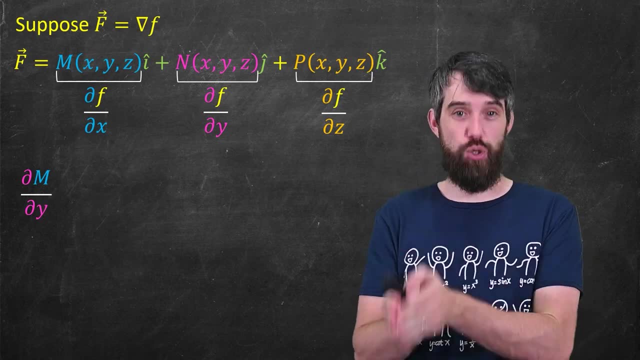 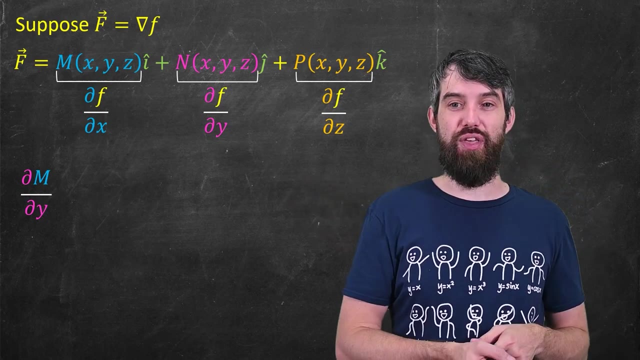 respect to x. n is the partial of f with respect to y and the p is the partial of f with respect to z. Let me consider the partial derivative of m with respect to y. Now, we just said that m was the partial derivative of f with respect to x. So, really, what this is saying is: I'm going to do two. 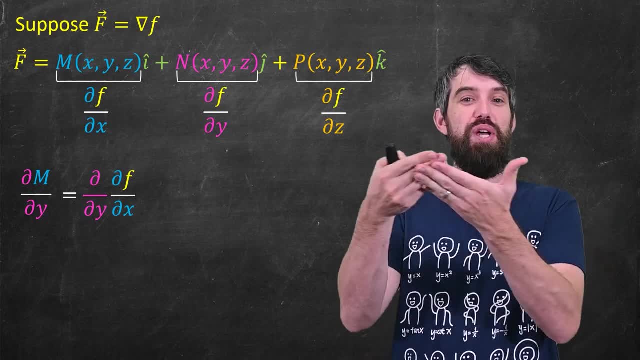 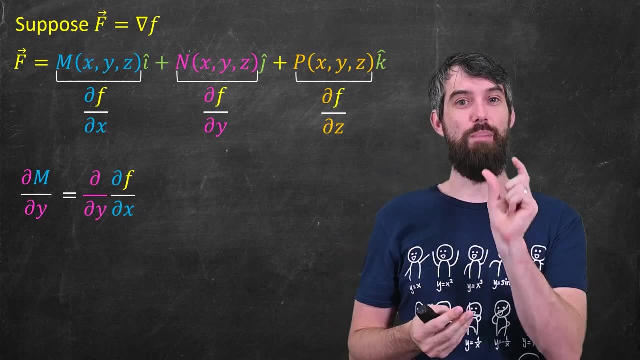 things. I'm going to take the partial derivative of f with respect to y, of the partial derivative of f with respect to x. Now we get to see another trick that we've seen back in multivariable calculus, namely about commuting mixed partials. That is as long as our f is sufficiently nice. 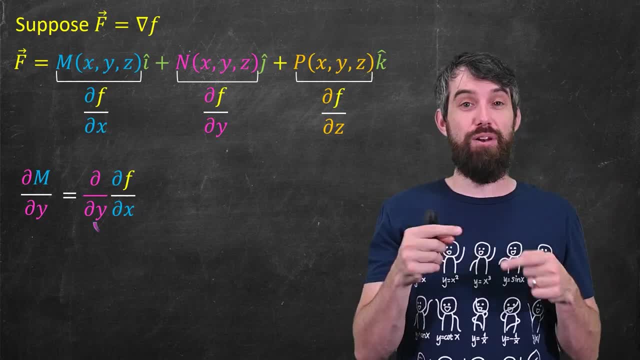 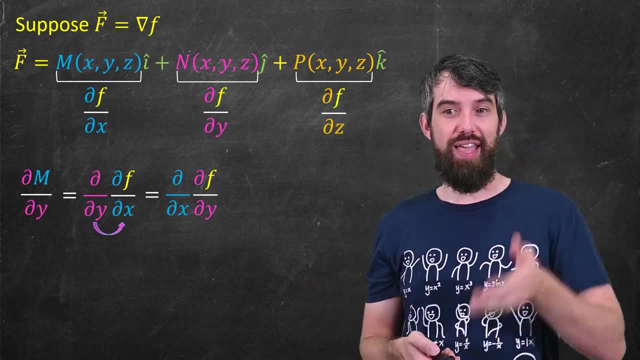 it needs to have the mixed partials being continuous. then I can switch it up. I can rewrite this as the partial, with respect to x, of the partial of f with respect to y. I've just changed the order- And then this can be reinterpreted as the partial derivative of x of n. 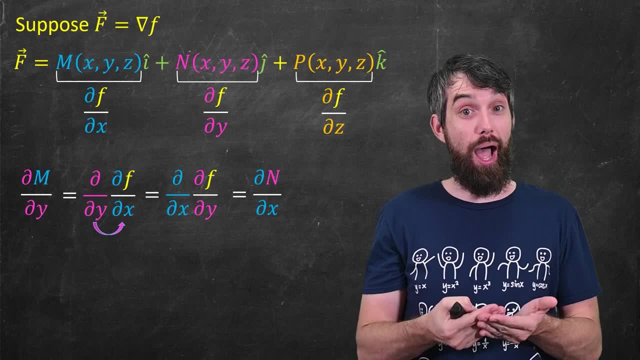 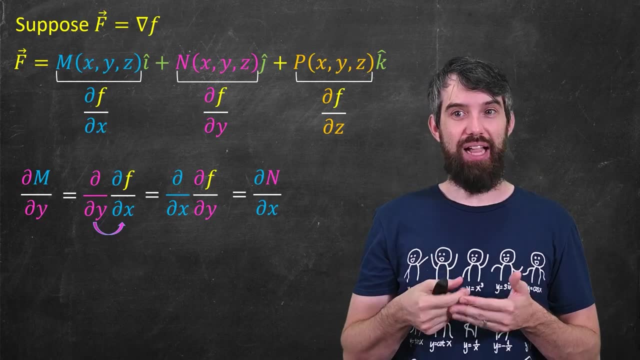 because n was the partial of f with respect to y. So the statement at the end is: the partial of n with respect to y is the partial of n with respect to x. I can do the same thing by comparing other pairs like the partial of n with. 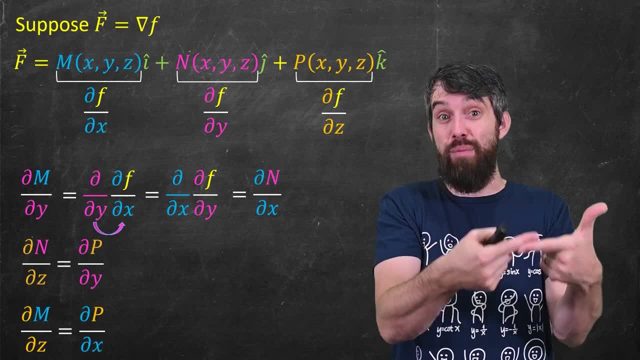 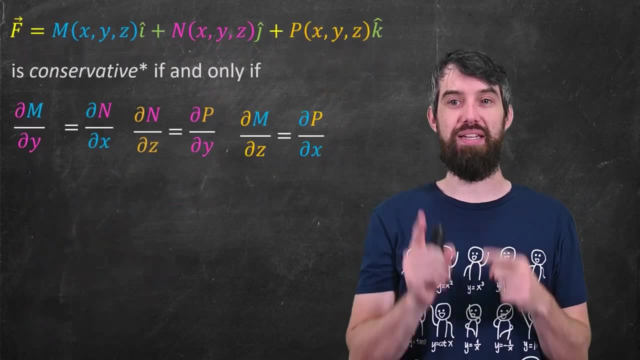 respect to z is like the partial of p with respect to y. or I can just say that the partial of m with respect to z is like the partial of p with respect to x. So I have these three different equalities here. I can put them all together and that is my test. The field is conservative. 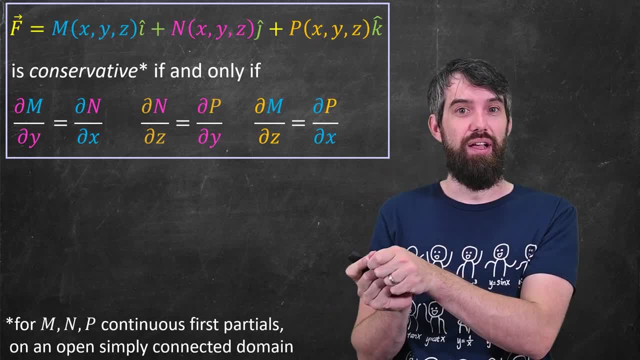 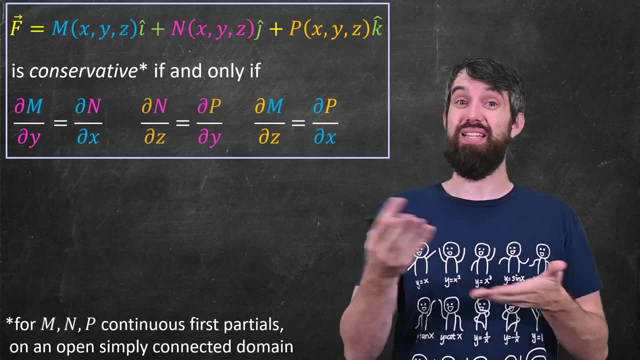 if and Krishna- Yeah, I can question it. the angle a, then these three different partial derivative equations are true. So take those six partial derivatives, which might sound like a lot, but partial derivatives are easy. Like you can do that really, really quickly. 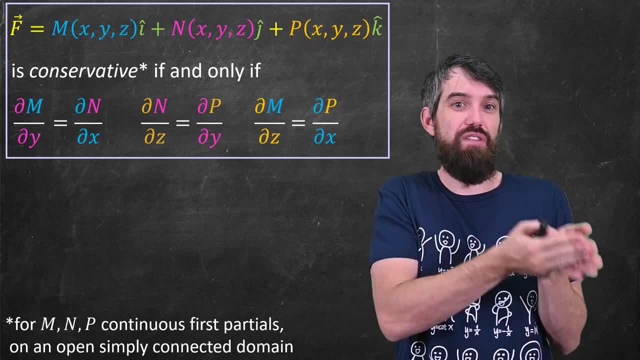 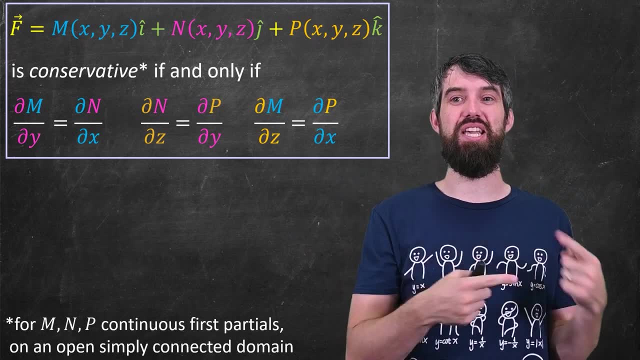 So it's a fast test. Take those six partial derivatives, see if those equations are all equal. and if all three of them are equal, then it's a conservative field. By the way, if you look at these, you can sort of see a bit of a pattern to it. 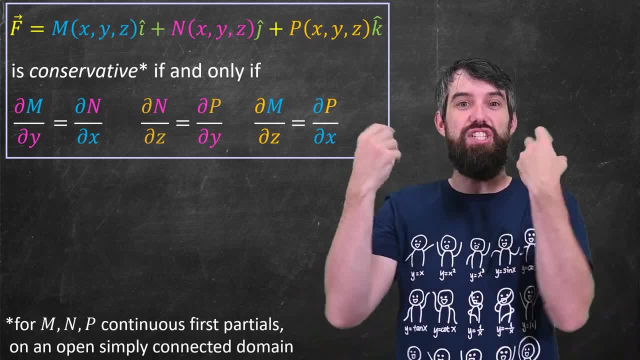 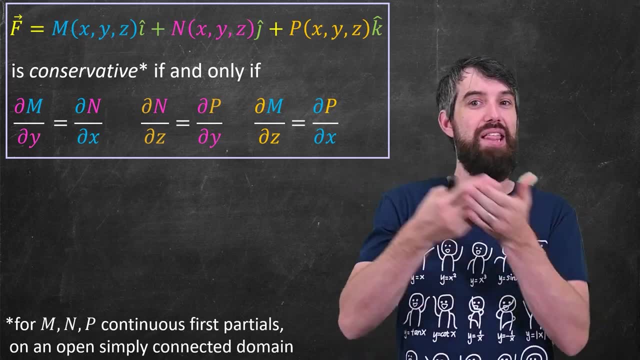 Basically, you've got the three different components: the m, the n and the p. You take any two of them, then you're comparing the derivatives, sort of of the same components as the two that you chose, Like if you chose the j-hat and the k-hat component. 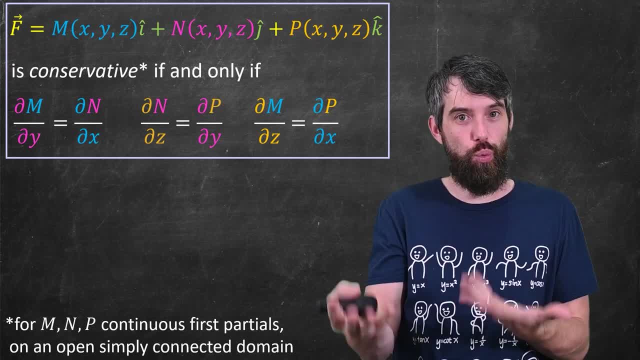 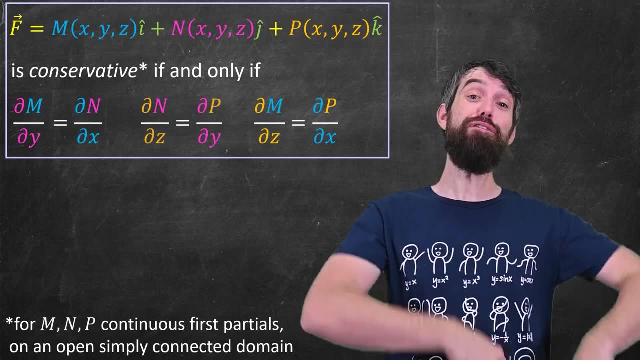 then you want to play around with the partial derivative y and z as well. Nevertheless, there's a bit of a pattern to easily memorize these. Now, I've only proven the one direction. I've proven that if it's conservative- namely, it can be written as the gradient of a potential function. 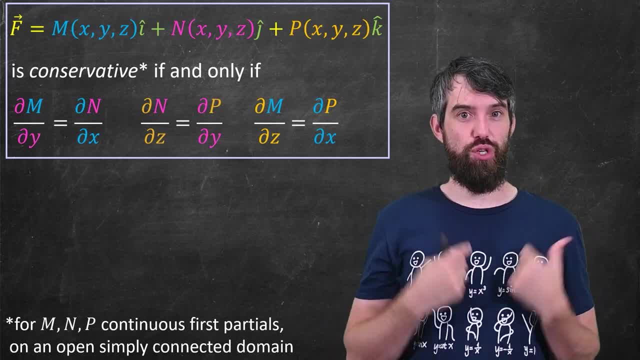 then these three things are true. The other direction works as well. In fact, that's needed for this to be a test. It has to be the case that when you have these partial derivatives, you also have to be able to do the same thing.